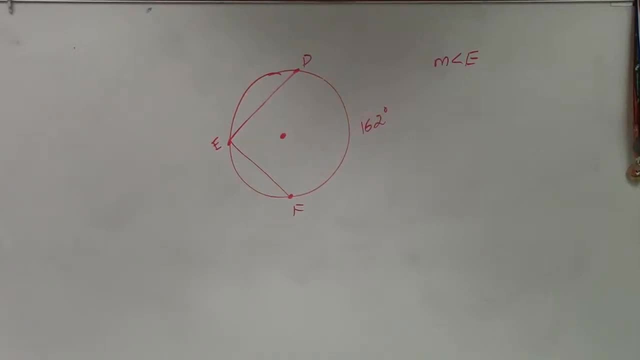 Or the people that they're talking to doesn't know or is not going to remember. So one thing I want you guys to remember is what we talked about last class. we brought up the case. The first thing we talked about was a central angle. Remember. 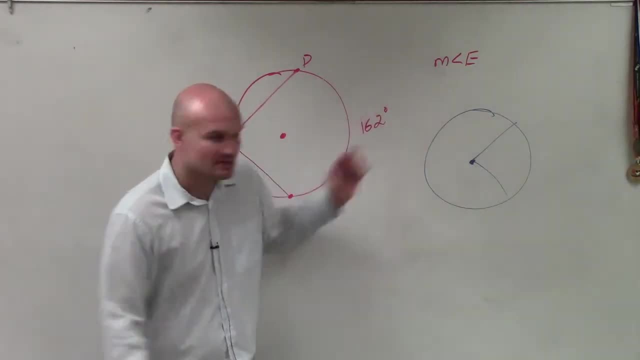 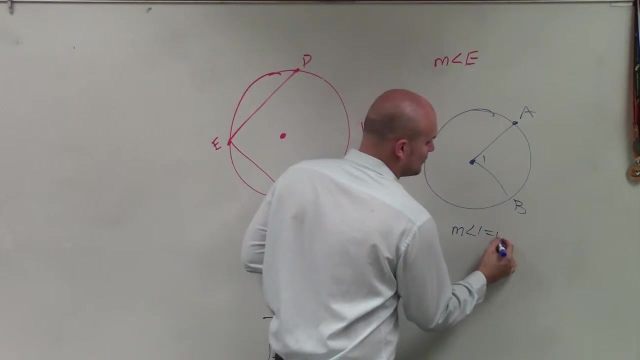 an angle that has the vertex at the center right. And if we have these two points, A to B, and we call this measure of angle one, we said the measure of angle one is equal to the measure of your arc AB. They're equal in measurements. So therefore, if I say that's 62 degrees, 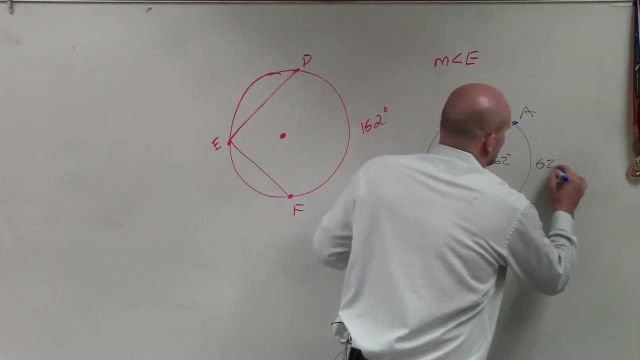 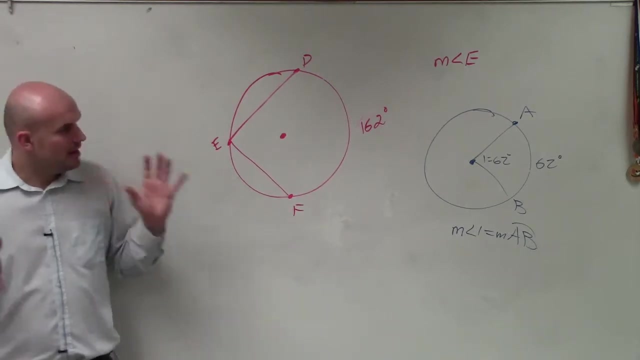 the arc measurement is also 62 degrees. right, That's what we're talking about: our central angles in the arc measure. They have the same measurements. Then, last class period, for your notes for this homework, we talked about inscribed angles. And if we did the exact same. 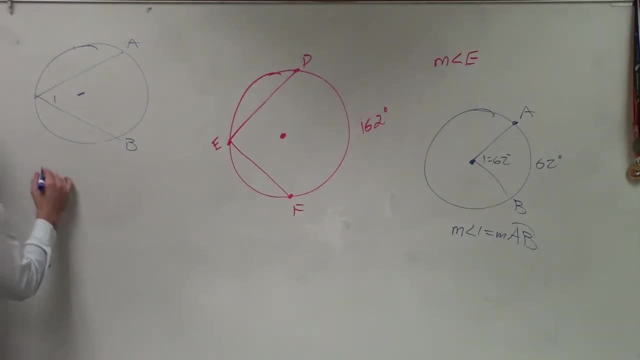 points and angle with an inscribed angle. what was different, though, now, is the measure of angle. one was equal to one half the measure of my arc AB, So when you have an angle that is not at the vertex, you're not at the vertex, You're at the vertex, You're at the vertex, You're at the. 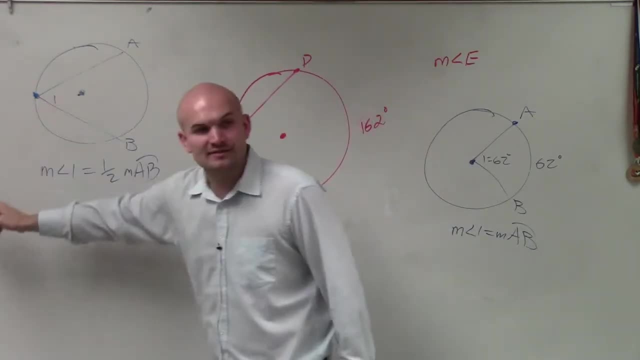 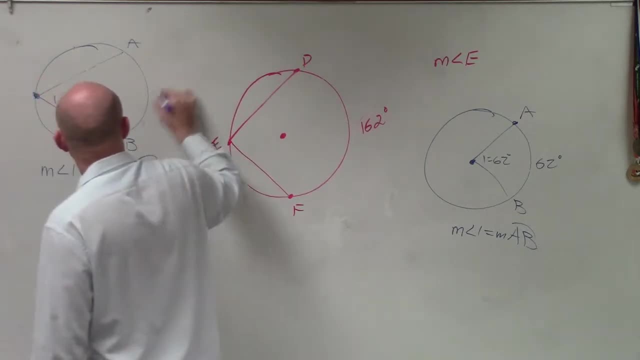 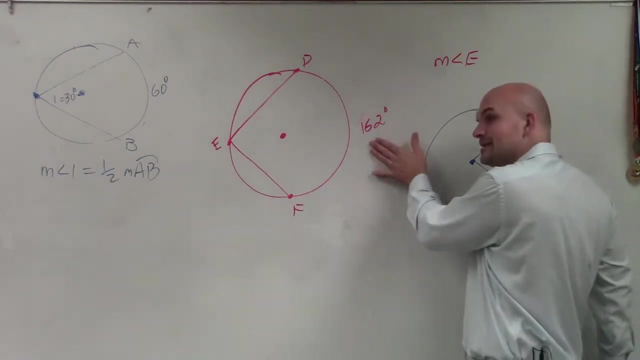 So if I said this was equal to 30 degrees, then my arc measurement would be 60 degrees. Does that make sense? That's what we learned last class period. So if I'm looking at this and I say 182, and I want to figure out what E is, then yeah, 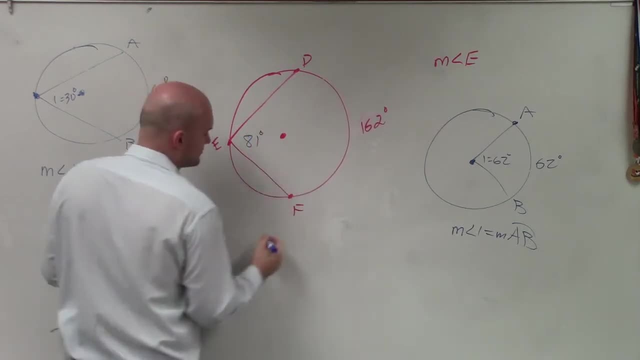 162 divided by 2.. E equals 1 half the measurement of my arc df. So I look at what is the measurement of my arc: It's 162 degrees. So it's 1 half times 162, which equals 81.. 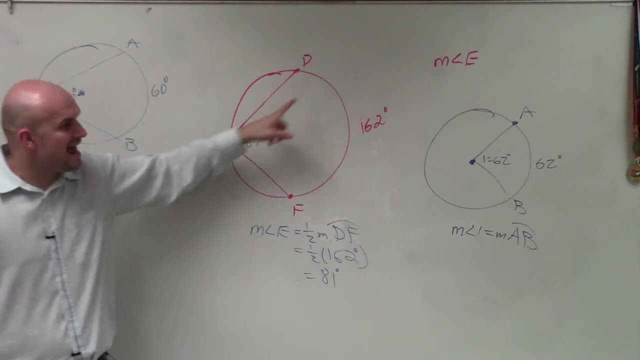 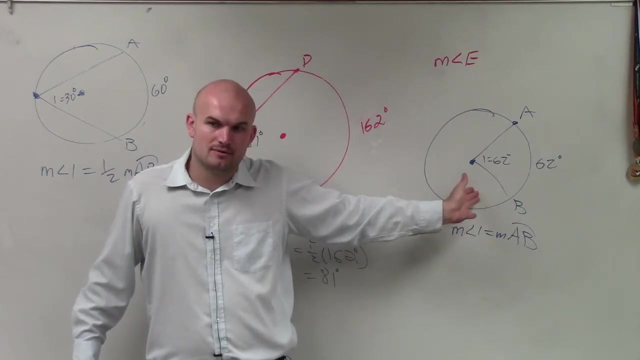 Remember the arc? when you have an inscribed angle, it's half of what it is. When it's a central angle, it's exactly the same. When it's, what exactly? On this circle? What did you say, Huh? 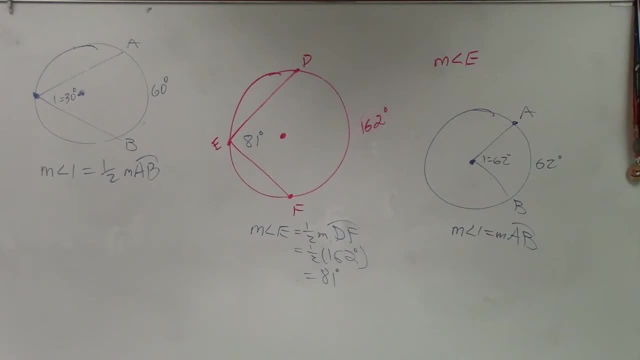 It's an inscribed angle when it's on the circle. No, you said inscribed angle is half, Half the arc measurement. What's the angle that you said? Central angle, which is exactly the same. So is this one like, like? 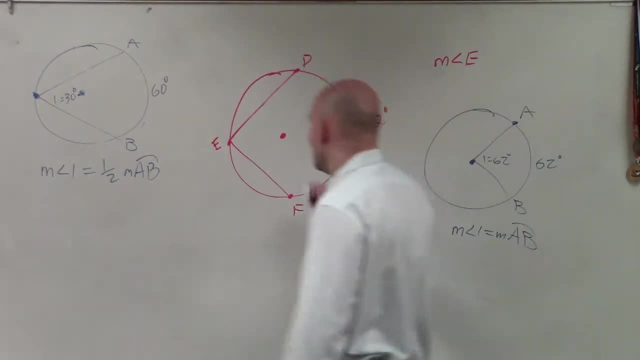 at this and I say 182 and I want to figure out what E is. then yeah, 162.. 162 divided by 2.. E equals one half the measurement of my arc DF. So I look at what is the measurement of my arc: it's 162 degrees, So it's one half. 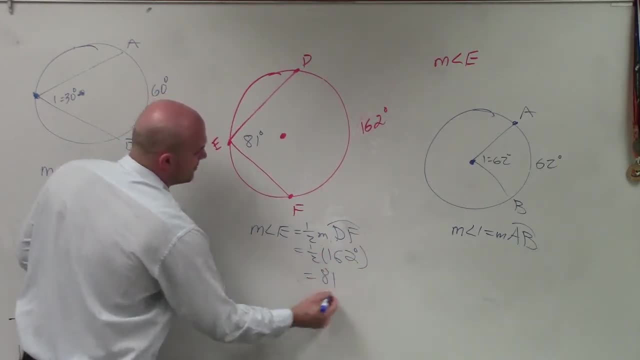 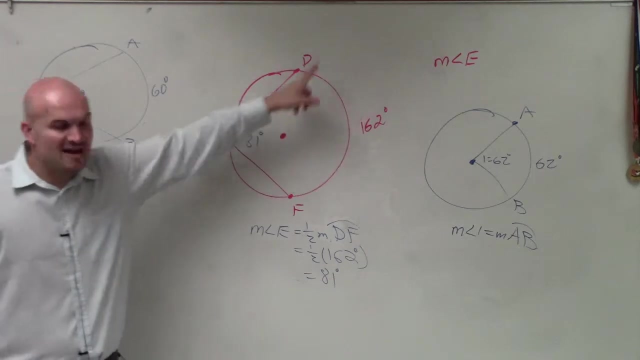 times 162, which equals 81.. Okay, Remember the arc. when you have an inscribed angle, it's half of the arc. So if I look at the arc, it's 162 degrees. So it's one half times 162, which equals 81.. 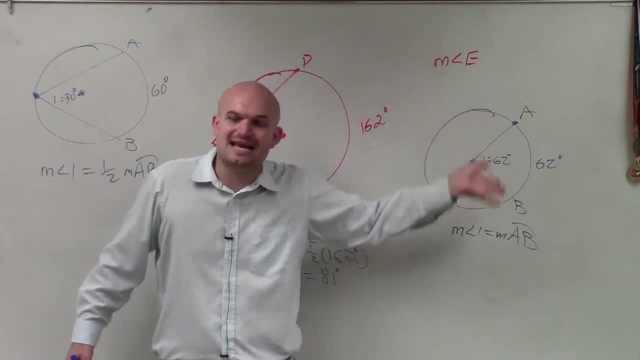 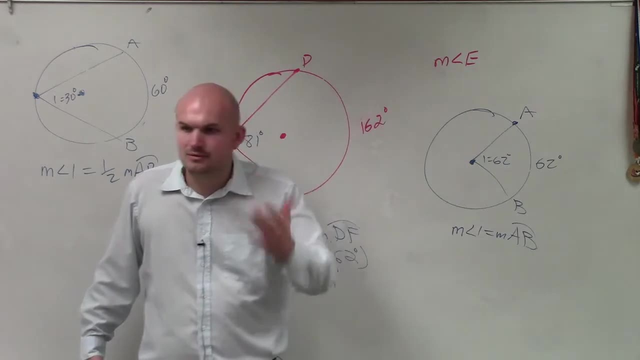 So it's one half times 162, which equals 81.. So what is exactly the measurement of what it is? When it's a central angle, it's exactly the same When it's what exactly On the circle? what did you say? 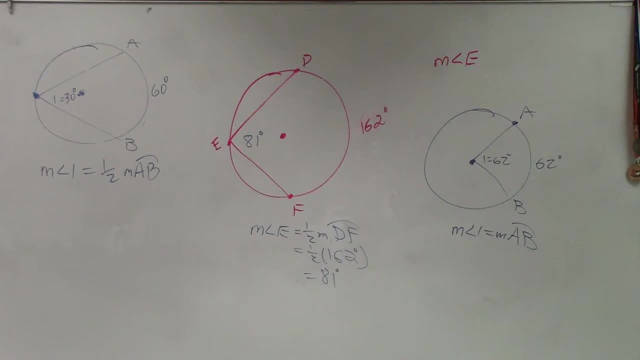 Huh, It's an inscribed angle when it's on the circle. When you said ins crimes, it was half the Half the arc measurement, Which is exactly the same. Central angle, which is exactly the same. So this, what like what. 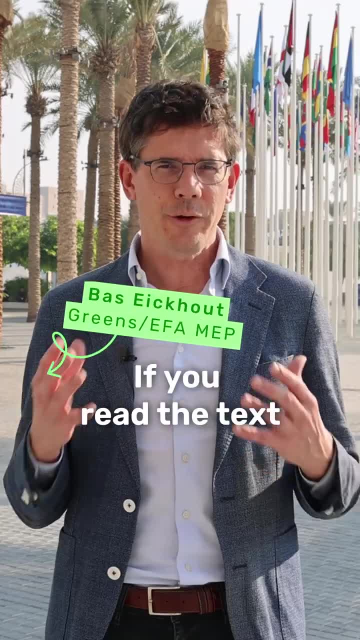 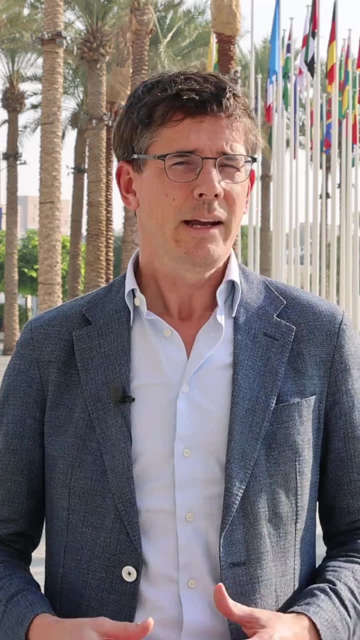 For the first time ever, we are marking the end of fossils. If you read the text- and it's clearly indicating that we need to transition away from the fossils, with an endpoint by 2050, it very clearly shows that the world has made a very big step here in Dubai. 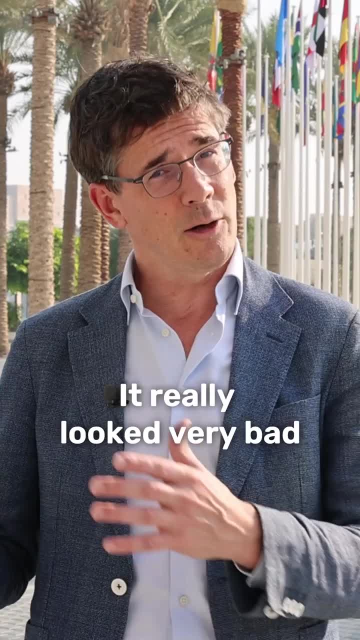 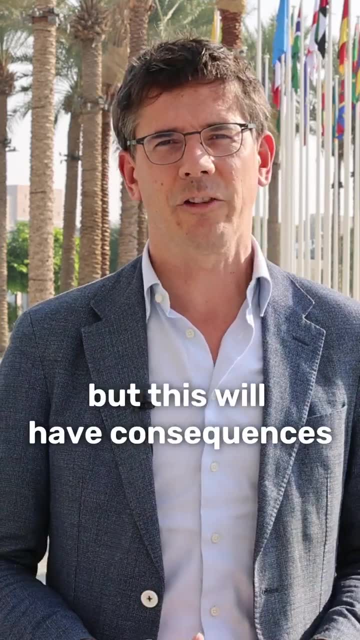 It could have been much stronger, certainly on phase-out. It really looked very bad a couple of days ago, but now we can mark an end of fossils in the energy system. but this will have consequences for investor choices And this must have big consequences for the European debate on 2040,. 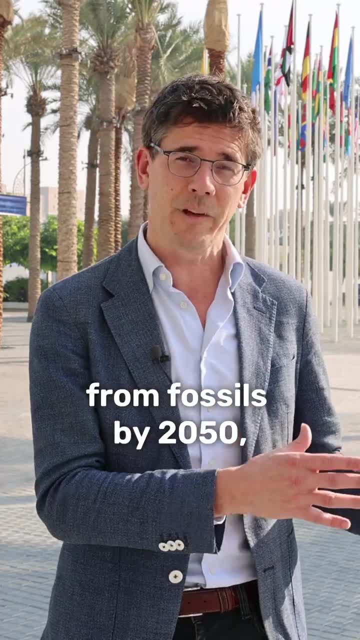 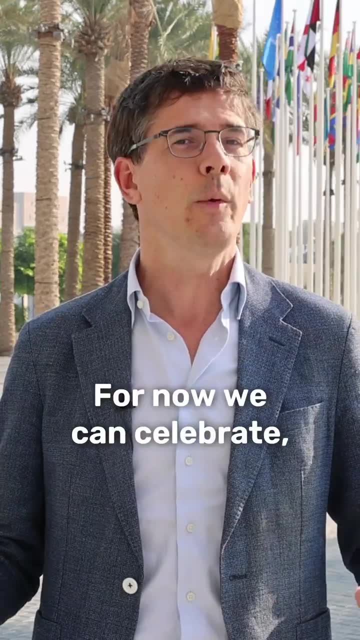 because if the world is transitioning away from fossils by 2050, this means that in 2040, Europe needs to be out of fossils in its energy system. For now, we can celebrate, but a lot of work needs to be done and needs to be translated. 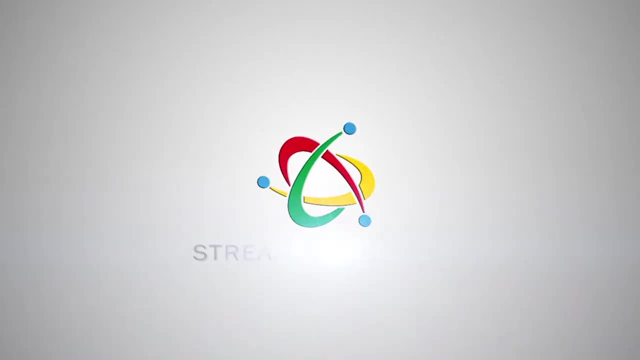 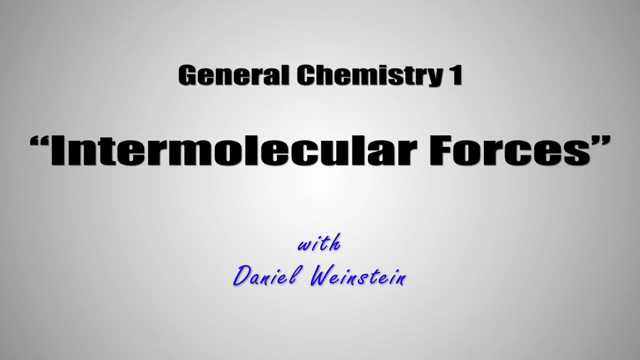 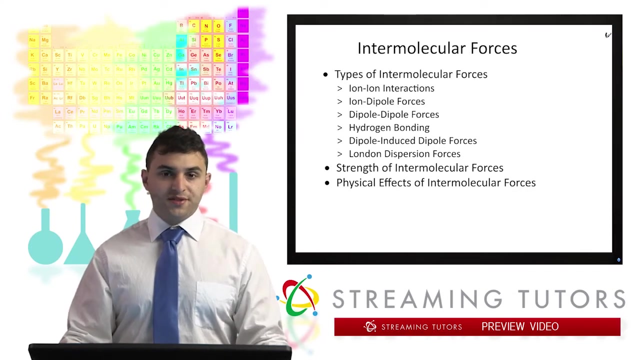 Hello, welcome back to General Chemistry. I, My name is Daniel, and in this video we're going to be looking at what's called intermolecular forces. So in the previous few videos we've been looking at the bonding between atoms within a molecule, and that's what's known.